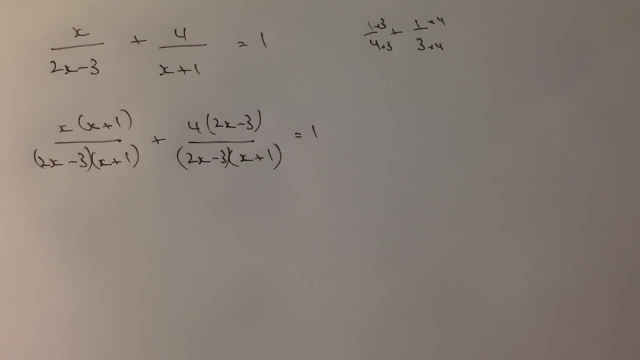 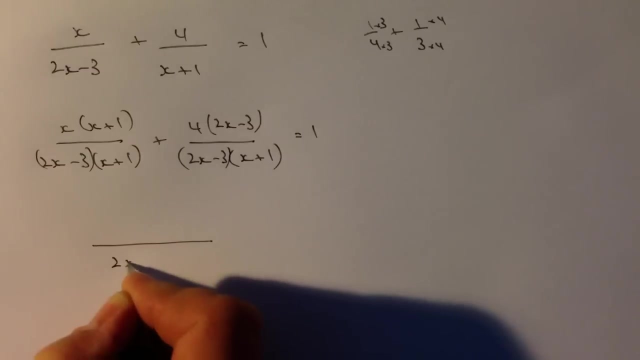 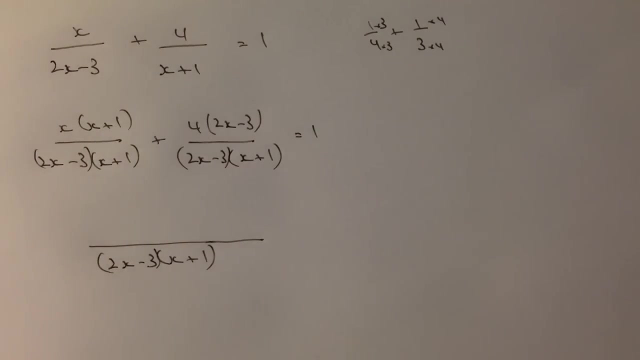 So it gives us now the ability to have this lowest or this common denominator, And I'm just going to write that out at the bottom- as being 2x minus 3 multiplied by x plus 1.. Now it's a case really of dealing with the top numbers. 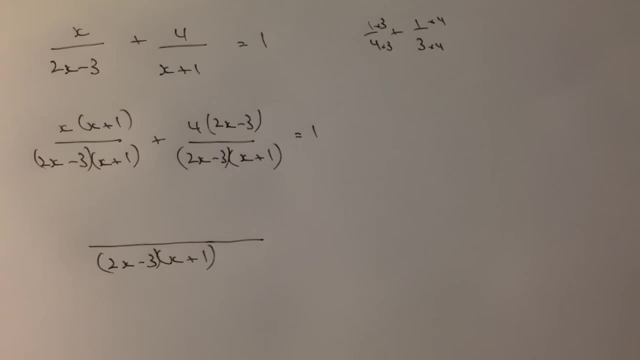 And this is where it does get a little bit tricky. But hopefully you'll be able to follow what I'm doing here, So I'm going to multiply these out first. So the first one I've got is x times x, which is going to give me x squared. 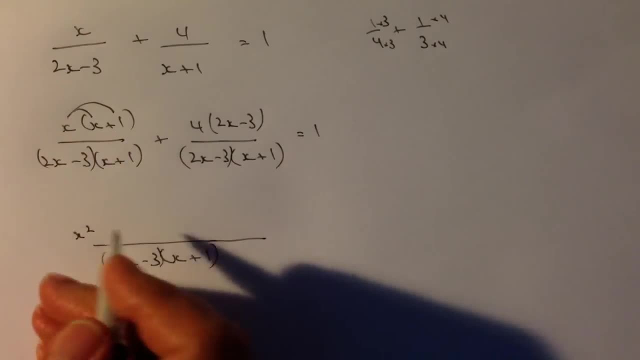 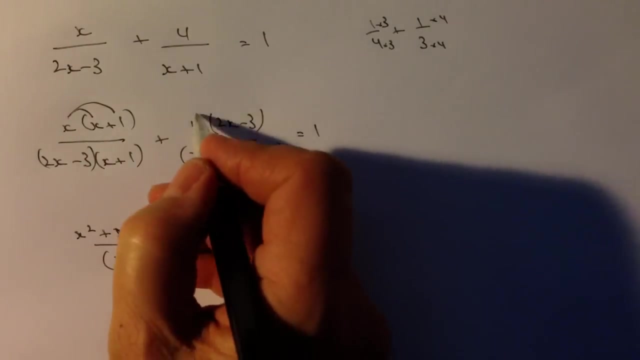 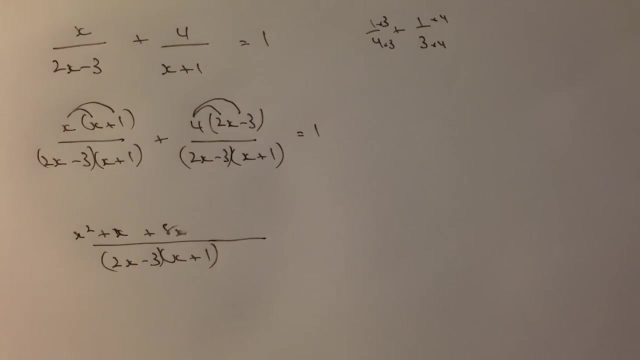 The second one I've got Is x times 1,, which is going to give me plus x. Then, on the second fraction, I've got 4 times 2x, which is going to give me 8x. And on the last bit of it, I've got positive 4 times minus 3, which is going to give me minus 12.. 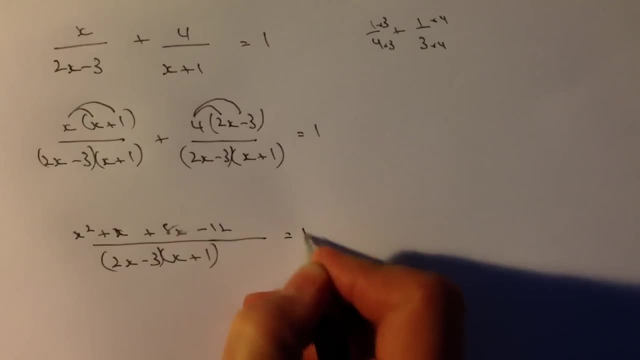 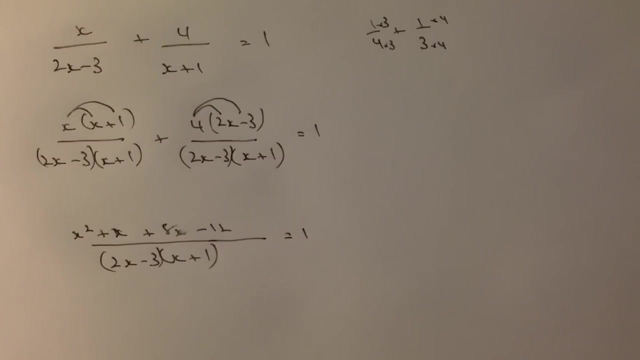 And don't forget that when we've done all of that, it still equals 1.. OK, so from here on in, really, it's just a case of tidying everything up And working out the two values of x. So the first thing I'm going to do is I'm going to write this just a little bit tidier, as x squared plus 9x minus 12.. 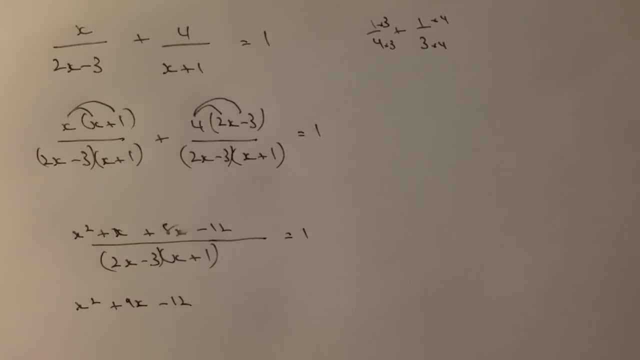 OK, so that's the top bit. The second bit I'm going to write as equal to this, But rather than having it this side of the equal sign, I'm going to multiply both sides through by 2x minus 3.. Brackets x. 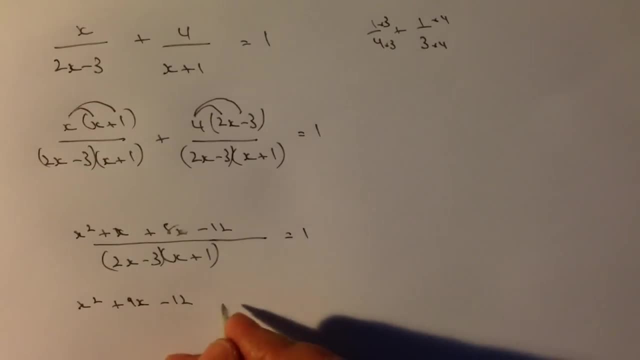 Plus 1.. That gets rid of this problem bit and puts it over here. So that's going to be equal to 2x minus 3 times x plus 1.. OK, so this is where it just gets a little bit more in detail. 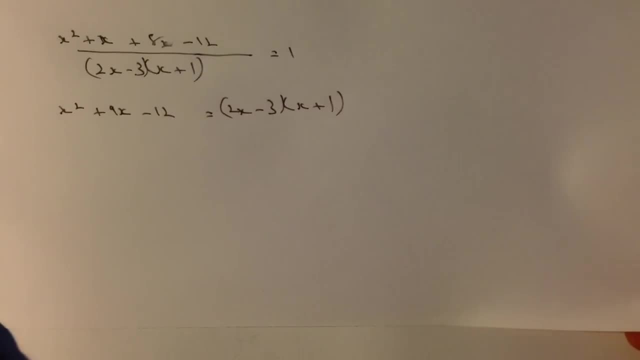 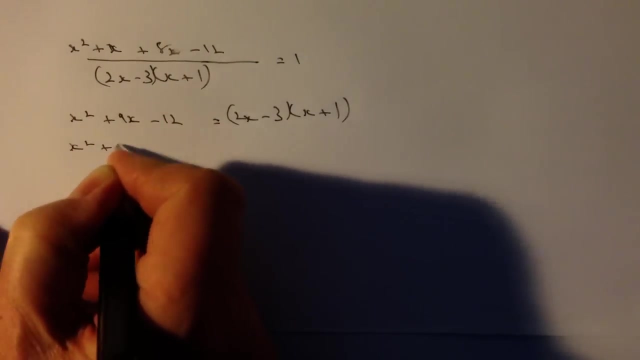 I'm going to move this page up and hopefully be able to follow it to this particular point. OK, so now we really need to just multiply out the brackets and solve everything. ie find the value of x, So I'm going to leave the left-hand side exactly as it is. 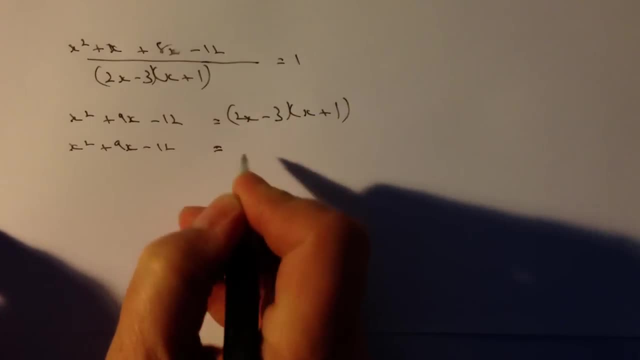 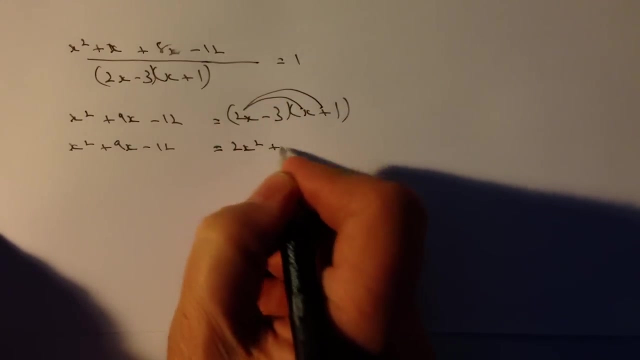 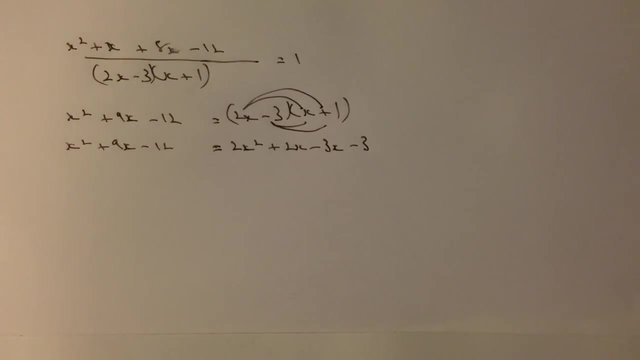 And with the right-hand side. I'm going to multiply out the brackets as 2x times x, which is 2x squared times 1, which is plus 2x minus 3x minus 3.. OK, now, in order to factorise this, I need to be able to bring everything over towards the right-hand side and make it equal to 0.. 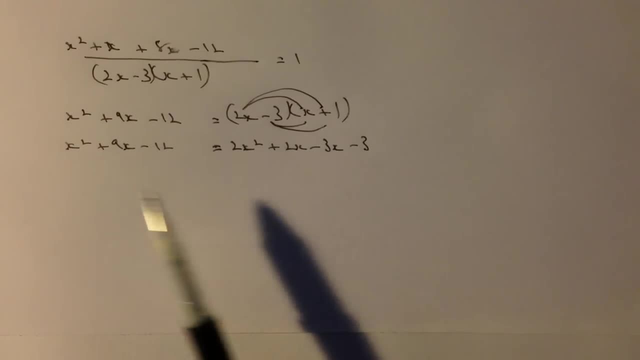 OK. So what I've chosen- the right-hand side- is because if I bring this x squared over to here, then it means I've got still a positive value. So this would be 2x squared minus x squared, So it becomes a positive value. 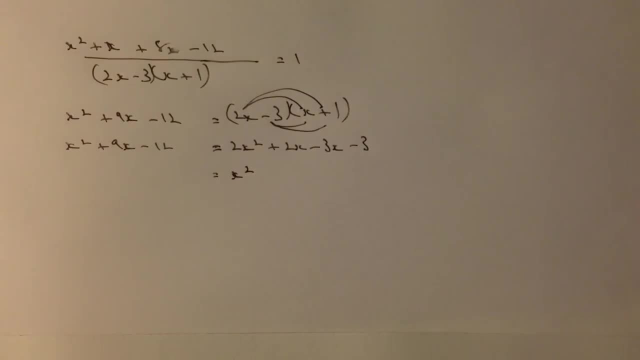 And it's really important with these that you make sure that when you're gathering your like terms, that you try to maintain positive values if you possibly can. OK, so this is going to be plus 2x, minus 3x. Well, that's going to be minus. 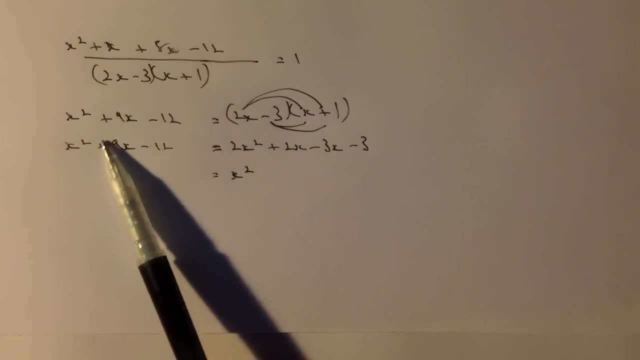 Minus x, And then on this side I've got plus 9x. Well, I'm going to bring this over. So that's going to be minus x, And this would be then minus 9x. So that's going to be minus 10x. 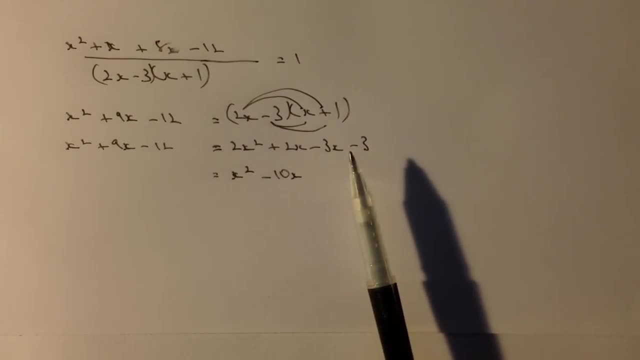 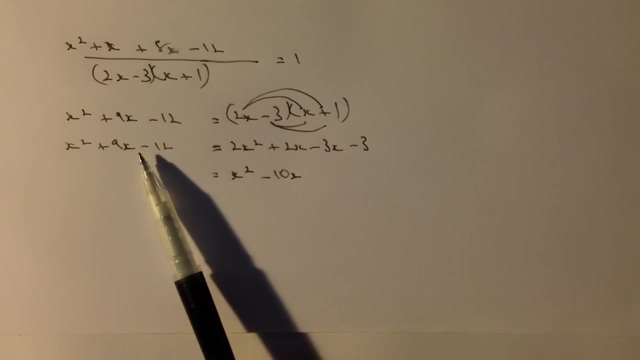 And then, finally, I've got minus 3 here And I've got minus 12.. Well, don't forget, when I bring this over to the other side, it's going to become a positive. So what I'm going to end up with is minus 3 plus 12.. 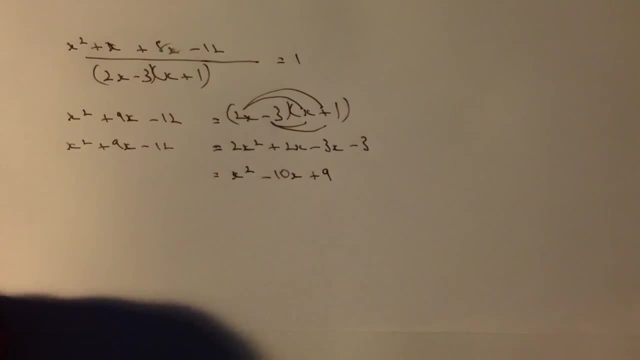 Which is going to give me plus 9.. OK, so we're now in a position where all of these equal to 0. And we can factorise this just by, in this particular case, trial and error. It's not always the case, I'm afraid. 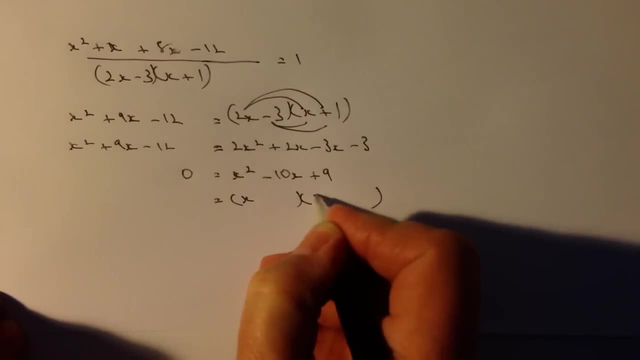 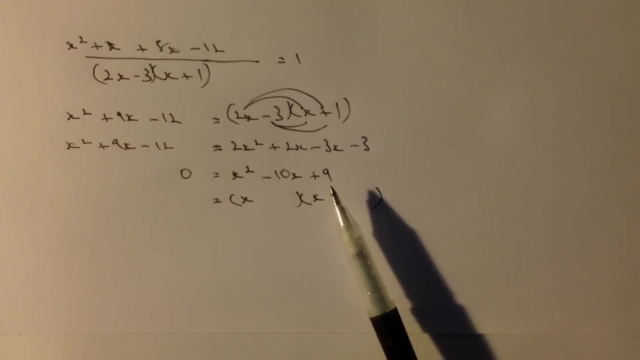 Sometimes you've got to use quadratic formula. But if you've had a bit of experience with factorising you'll be able to look at that and say the two factors of 9 that multiply together to make 9 will be either positive, So negative- 9 times positive 1, or negative- 9 times negative 1..